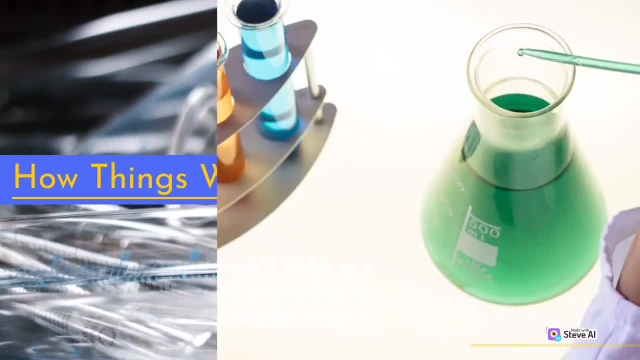 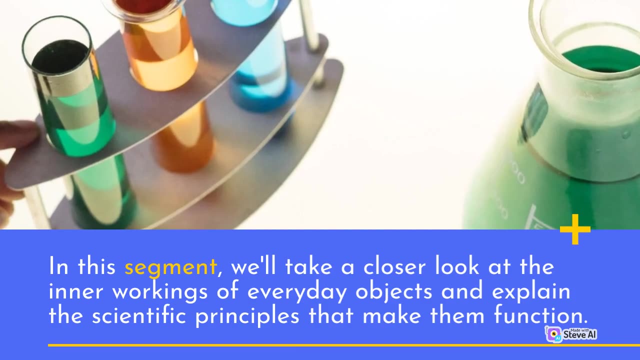 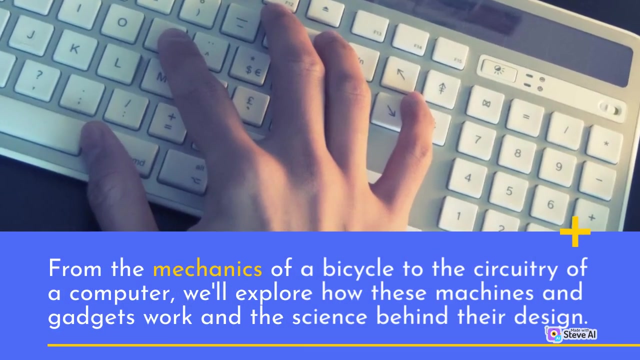 How things work. In this segment, we'll take a closer look at the inner workings of everyday objects and explain the scientific principles that make them function. From the mechanics of a bicycle to the circuitry of a computer, we'll explore how these machines and gadgets work and the science behind their design. 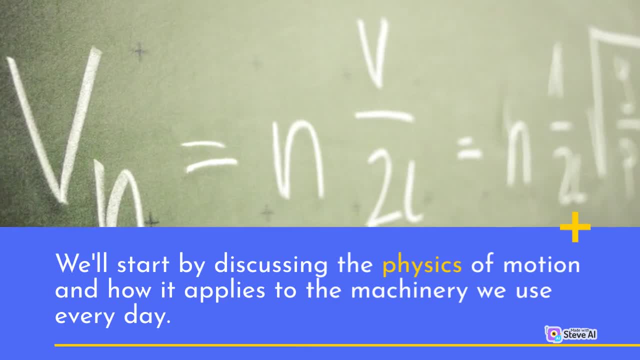 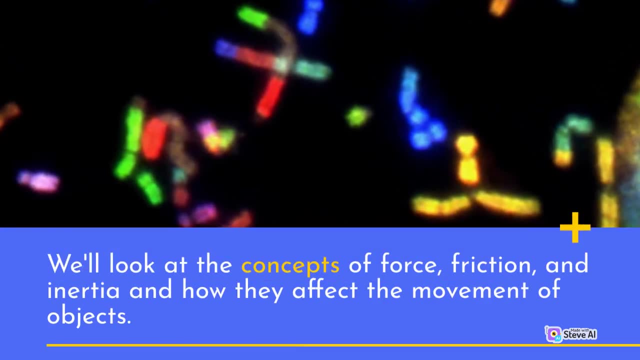 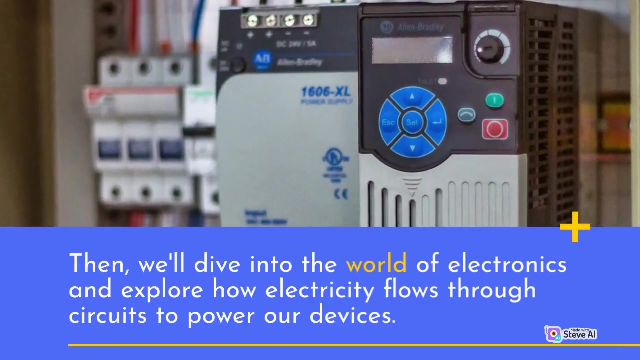 We'll start by discussing the physics of motion and how it applies to the machinery we use every day. We'll look at the concepts of force, friction and inertia and how they affect the movement of objects. Then we'll dive into the world of electronics and explore how electricity flows through circuits to power our devices. 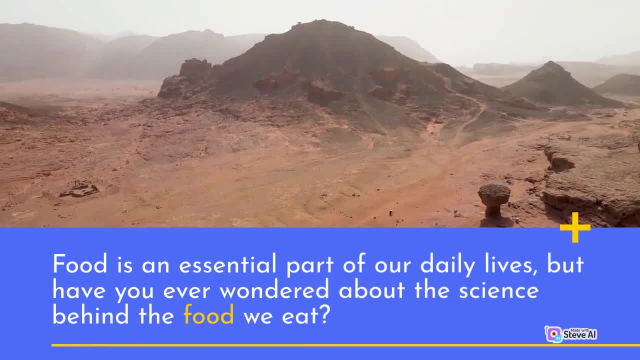 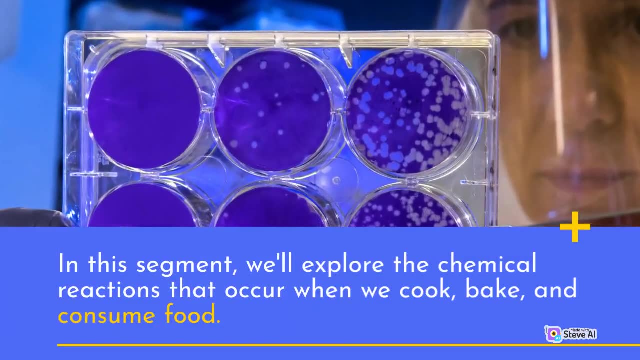 Food is an essential part of our daily lives, but have you ever wondered about the science behind the food we eat? In this segment, we'll explore the key to our everyday lives. In this segment, we'll explore the key to our everyday lives. 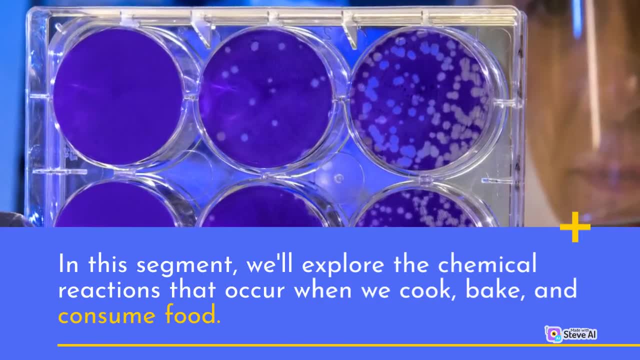 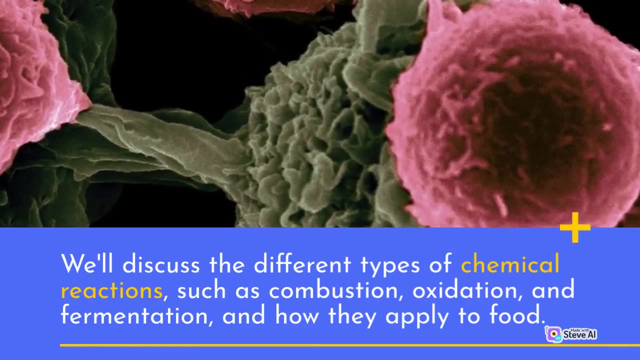 In this segment, we'll explore the key to our everyday lives: chemical reactions that occur when we cook, bake and consume food. We'll discuss the different types of chemical reactions, such as combustion, oxidation and fermentation, and how they apply to food. 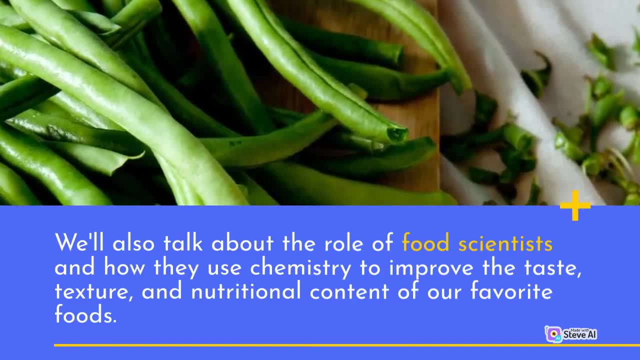 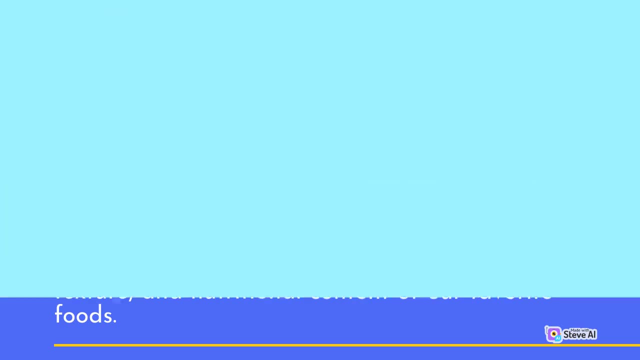 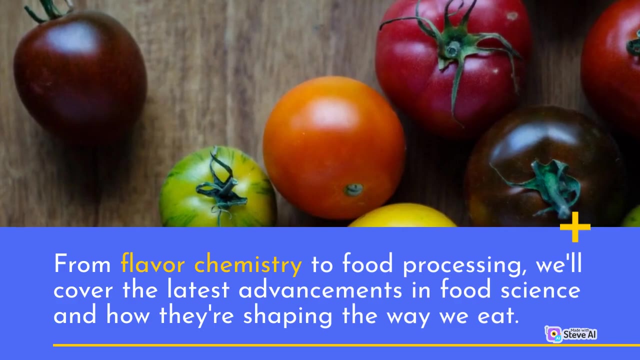 We'll also talk about the role of food scientists and how they use chemistry to improve the taste, texture and nutritional content of our favorite foods. From flavor chemistry to food processing, we'll cover the latest advancements in food science and how they're shaping the way we eat. 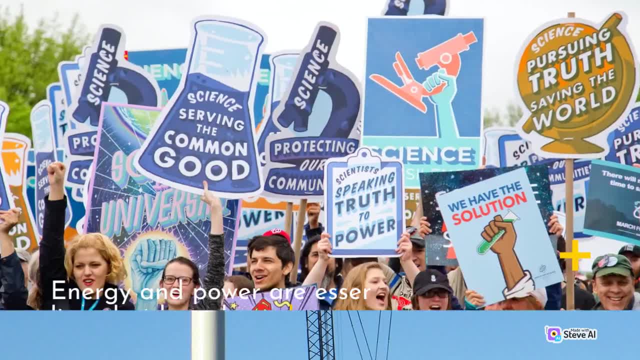 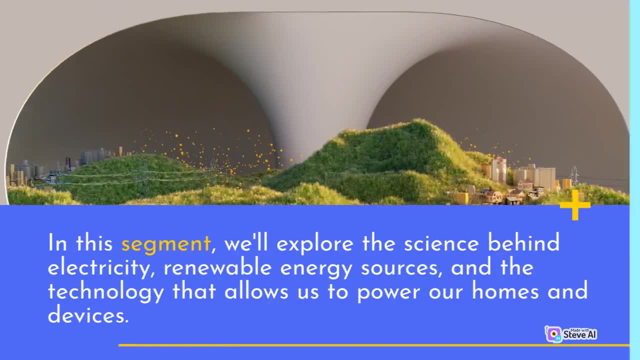 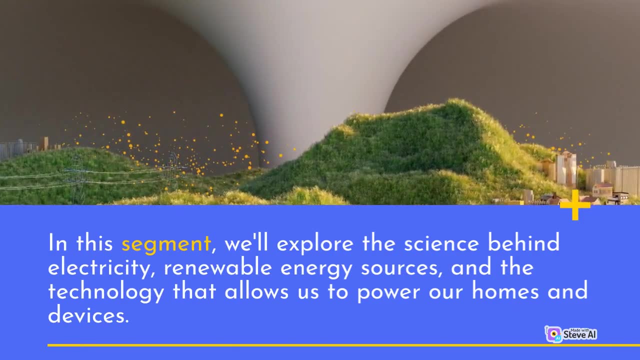 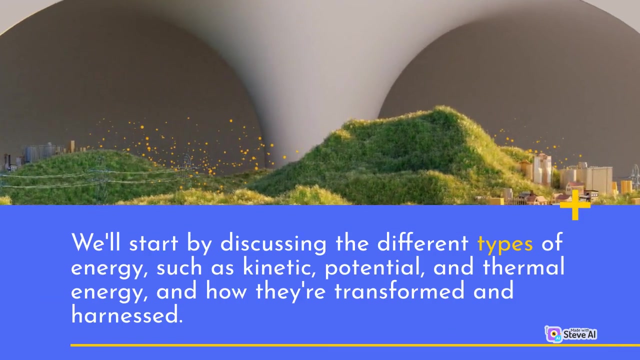 Energy and Power. Energy and power are essential to our modern lives, but how do we harness and use them? In this segment, we'll explore the science behind electricity, renewable energy sources and the technology that allows us to power our homes. We'll start by discussing the different types of energy, such as kinetic potential and 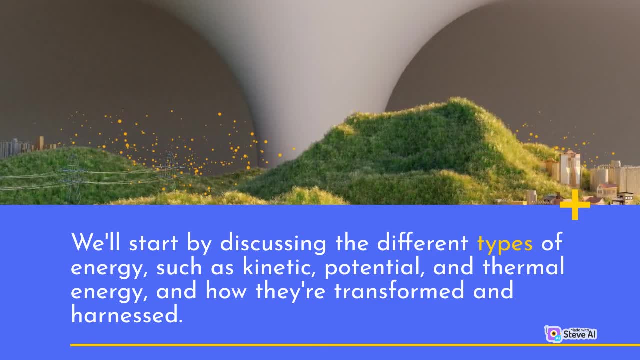 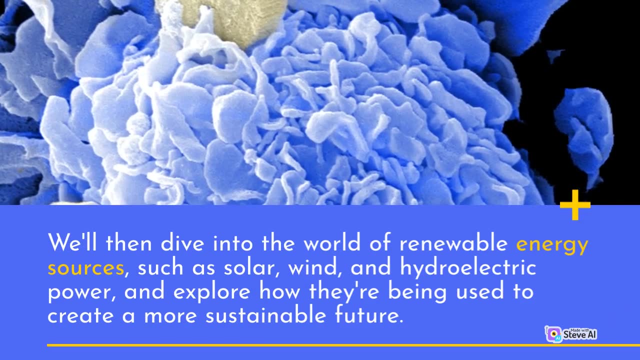 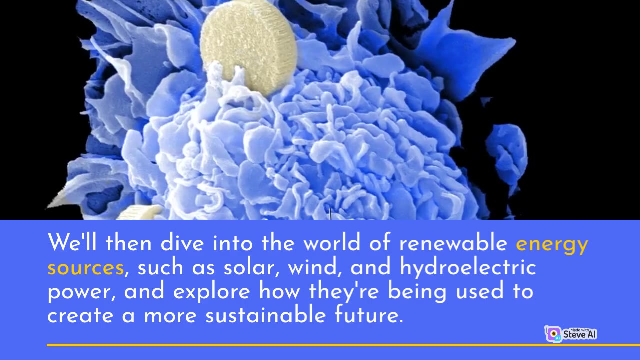 thermal energy and how they're transformed and harnessed. We'll then dive into the world of renewable energy sources, such as solar, wind and hydroelectric power, and explore how they're being used to create a more sustainable future. Finally, we'll discuss the latest advancements in battery technology and how they're being 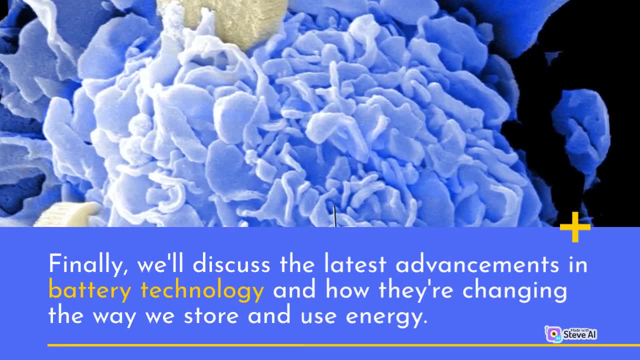 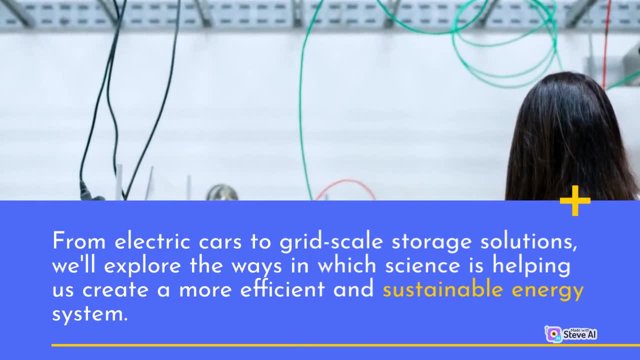 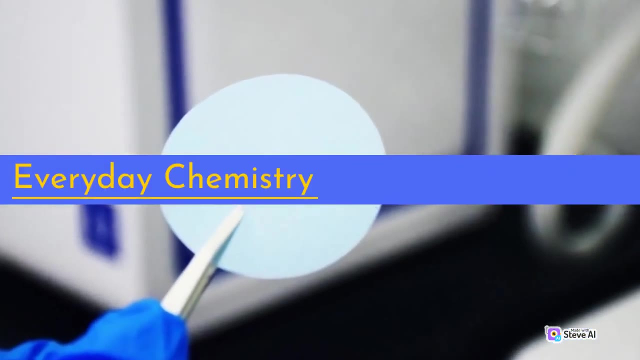 used and how they're changing the way we store and use energy, From electric cars to grid-scale storage solutions. we'll explore the ways in which science is helping us create a more efficient and sustainable energy system. Everyday Chemistry. Chemistry plays a huge role in our daily lives, from the products we use to the air we breathe. 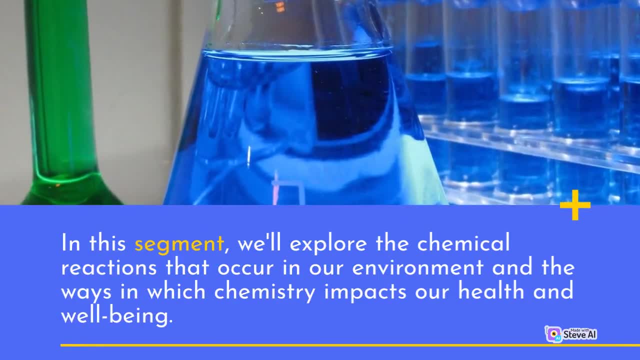 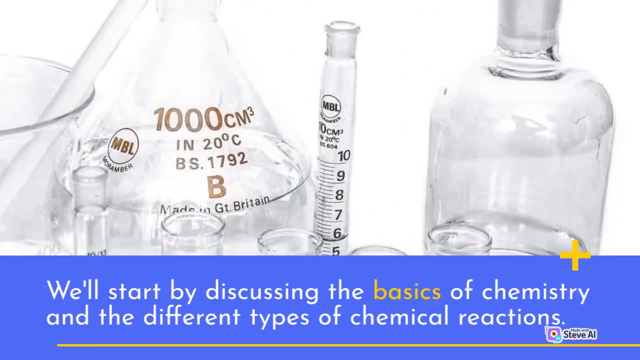 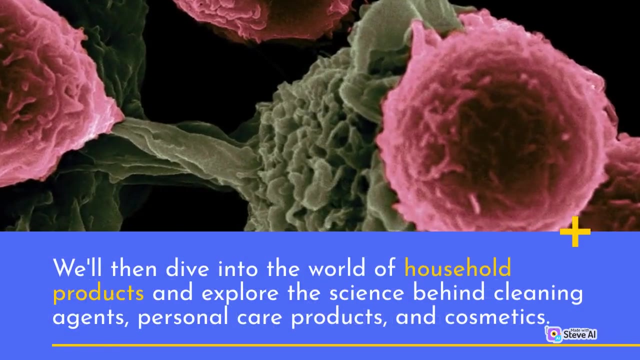 In this segment, we'll explore the chemical reactions that occur in our environment and the ways in which chemistry impacts our health and well-being. We'll start by discussing the basics of chemistry and the different types of chemical reactions. We'll then dive into the world of household products and explore the science behind cleaning. 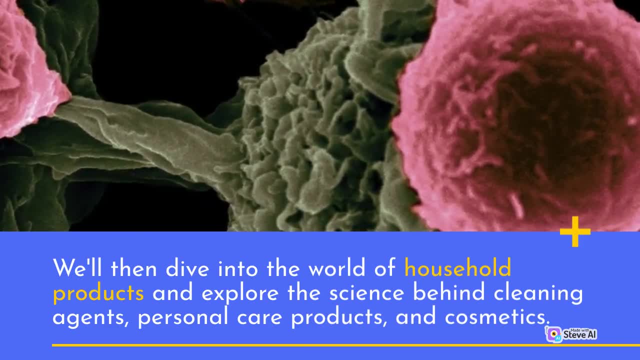 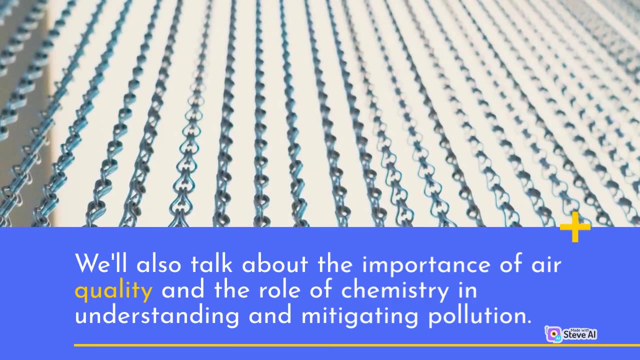 agents, personal care products and cosmetics. We'll also talk about the importance of air quality and the role of chemistry in understanding and mitigating pollution. Finally, we'll discuss the importance of air quality in our daily lives and the role of air quality in our daily lives. 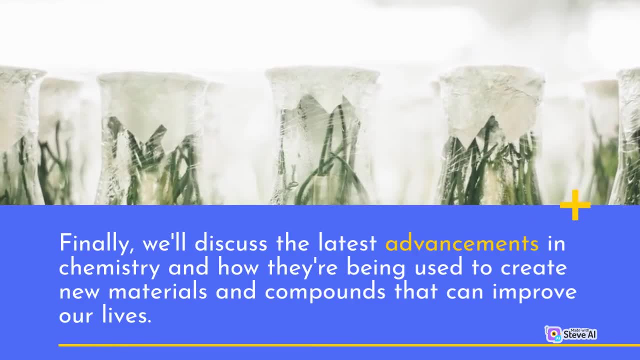 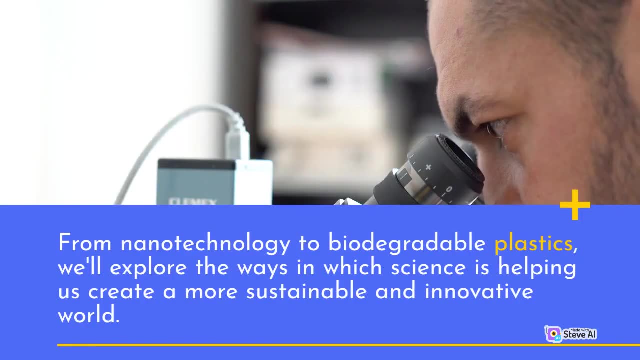 We'll also talk about the importance of air quality and the role of chemistry in understanding and mitigating pollution. We'll also discuss the latest advancements in chemistry and how they're being used to create new materials and compounds that can improve our lives, From nanotechnology to biodegradable plastics. 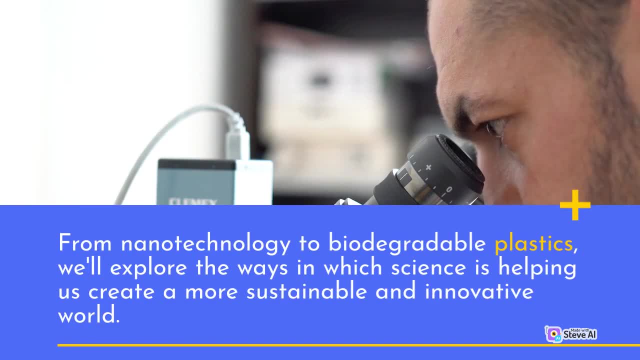 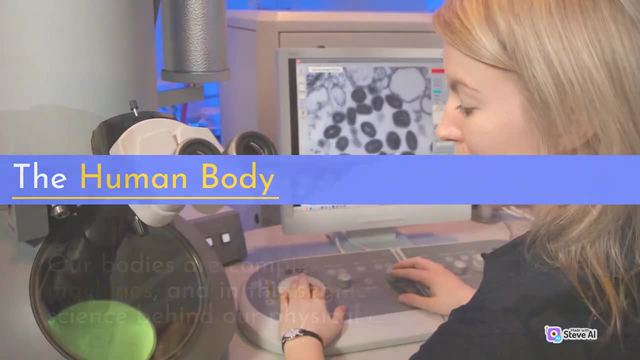 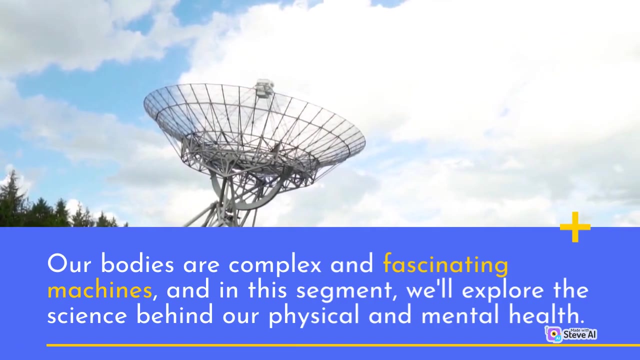 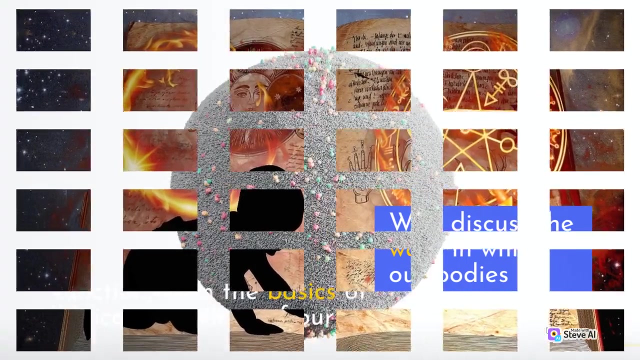 we'll explore the ways in which science is helping us create a more sustainable and innovative world. The Human Body, Our bodies, are complex and fascinating machines and in this segment, we'll explore the science behind our physical and mental health. We'll discuss the ways in which our bodies function, from the basics of cell biology. 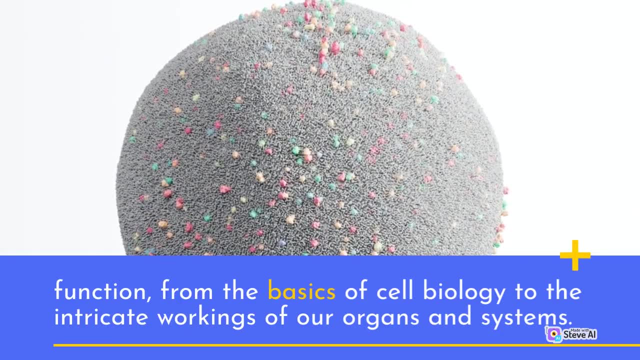 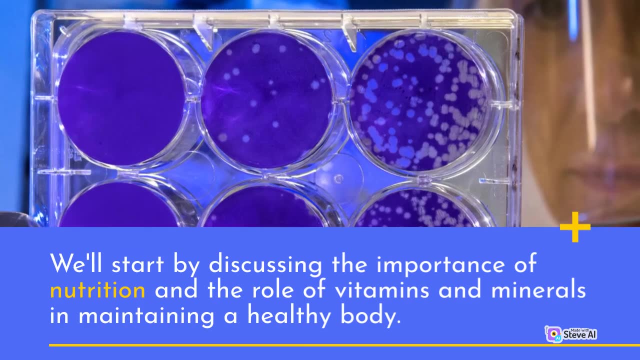 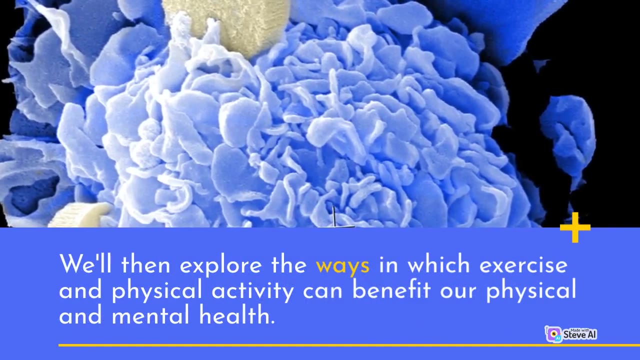 to the intricate workings of our organs and systems. We'll start by discussing the importance of nutrition and the role of vitamins and minerals in maintaining a healthy body. We'll then explore the ways in which exercise and physical activity can benefit our physical and mental health. 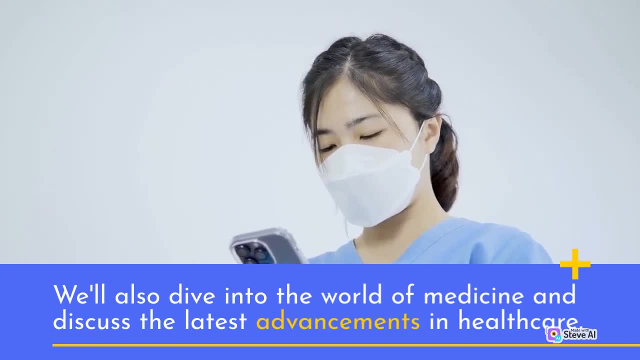 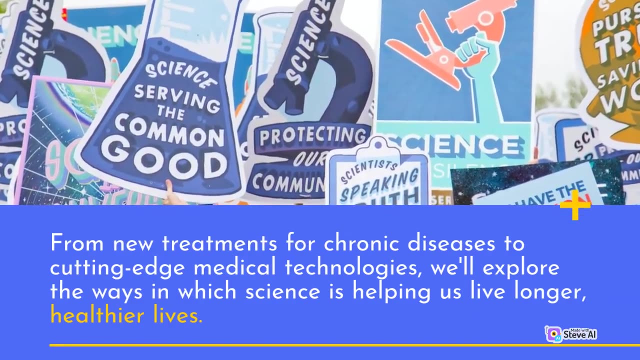 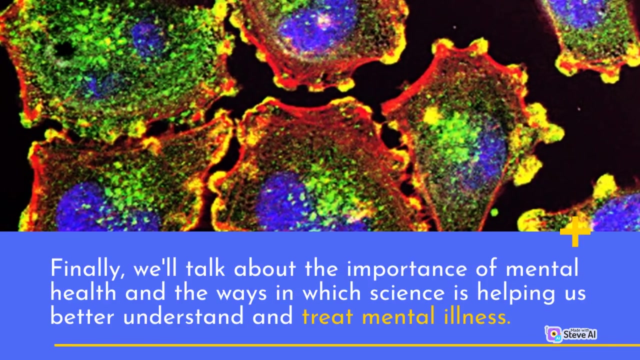 We'll also dive into the world of medicine and discuss the latest advancements in healthcare, From new treatments for chronic diseases to cutting-edge medical technologies. we'll explore the ways in which science is helping us live longer, healthier lives. Finally, we'll talk about the importance of mental health and the ways in which science 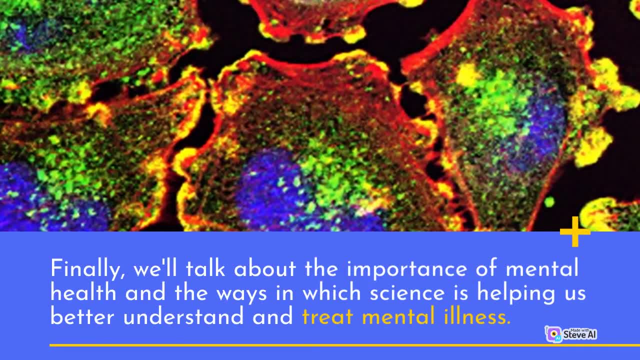 is helping us better understand and treat mental illness. From the latest advancements in psychotherapy to the role of neuroscience and psychology, we'll explore the ways in which our bodies function, from the basics of cell biology to the intricate workings of our organs and systems.